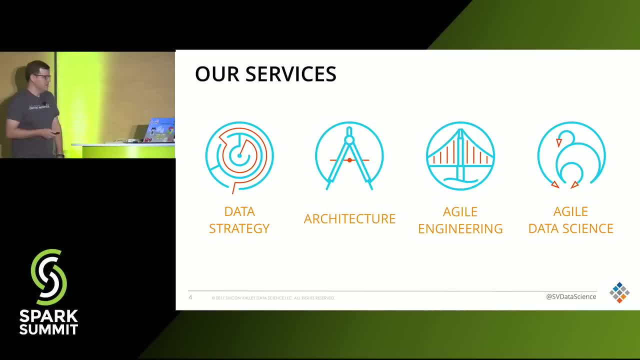 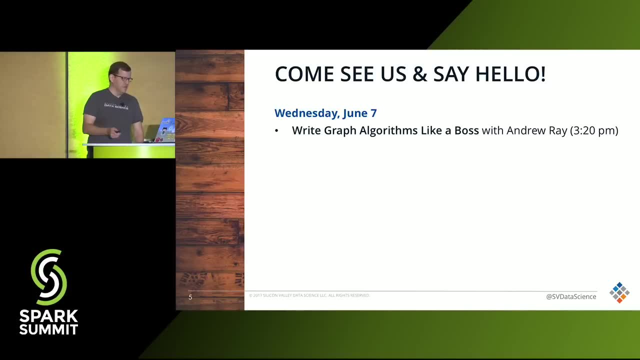 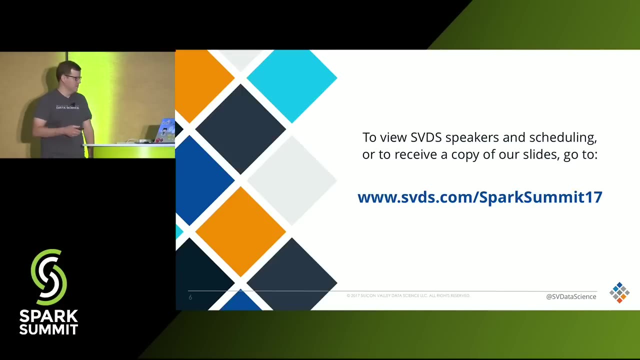 So we offer data strategy, architecture, engineering and agile data scientists. Okay, Also later this afternoon, I'm giving another talk on graph algorithms. If you're interested, come see us, And if you want to get copies of these slides or any of the other talks that we've done at Spark Summit, go to our website and you can put in your contact information and we'll send them out to you right away. 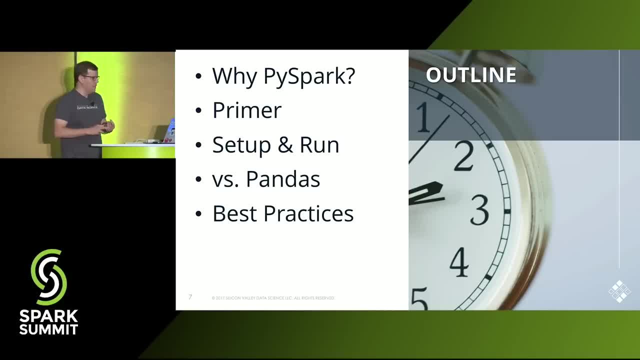 Okay. So what are we going to do today? We're going to talk about why PySpark. give a quick primer on Spark, how to get set up and running on your laptop, compare it to Pandas and then talk about some best practices. 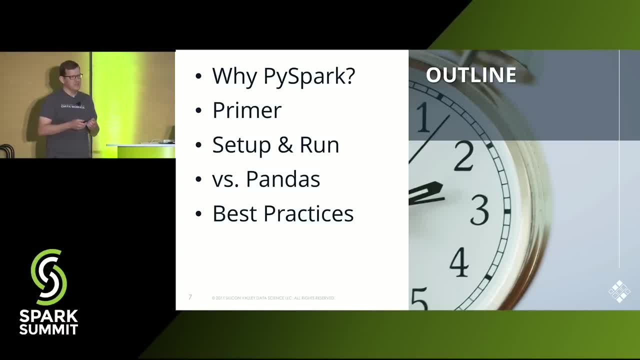 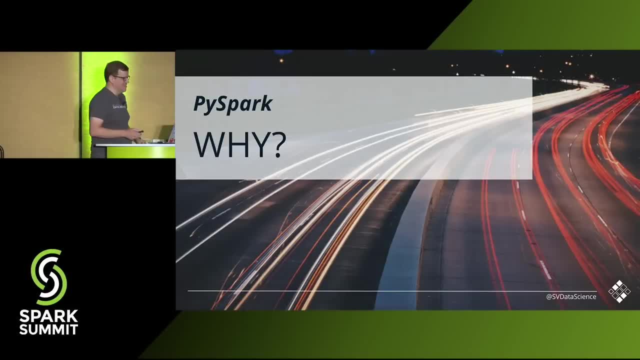 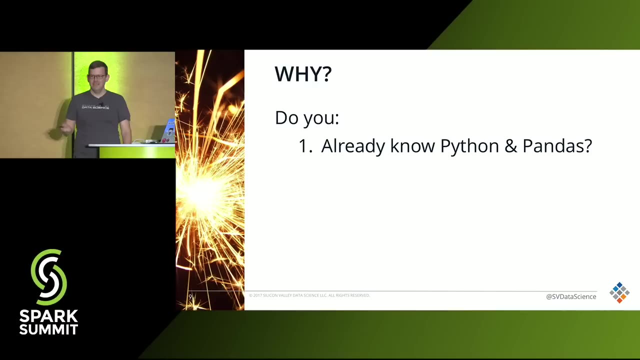 And so this is really a very much introductory talk. so if that's not what you're looking for, here's your chance to Okay, So why PySpark? Okay, Okay, So why do you already know Python and Pandas Love data frames, Want to work with big data? Okay, PySpark's the answer. It's what you're looking for. It is the answer to all of these questions. 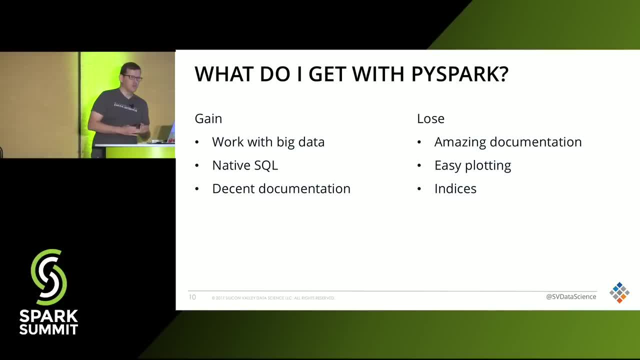 Okay, What do you get? You gain the ability to work with big data, very, very good native SQL support. decent documentation- Say decent, You lose, on the other hand, very amazing documentation. Pandas has been around a lot longer. it has really good documentation, has great plotting- PySpark does not- and support for indices. If you know a lot about Pandas already, that's the basis for DataFrames. it's all about indices. You don't have that there. 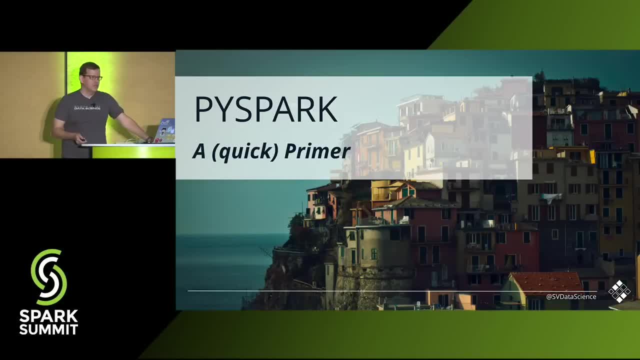 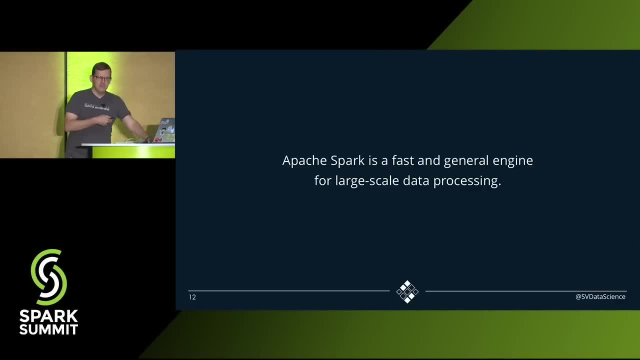 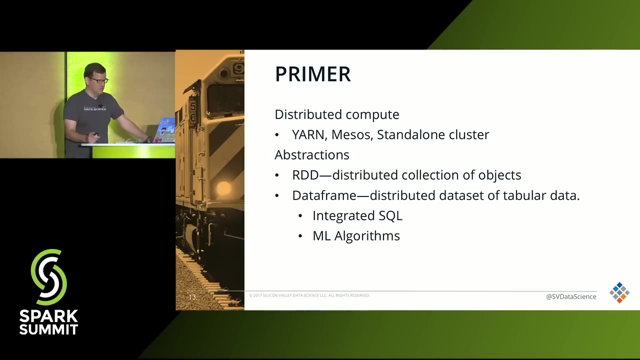 Okay, So let's give a quick primer on how PySpark works and Spark in general. So you've probably seen this blurb before. Spark is a fast general engine for large-scale data processing synopsis, So it runs on distributed compute, that is, Yarn, Mesos or a standalone cluster. 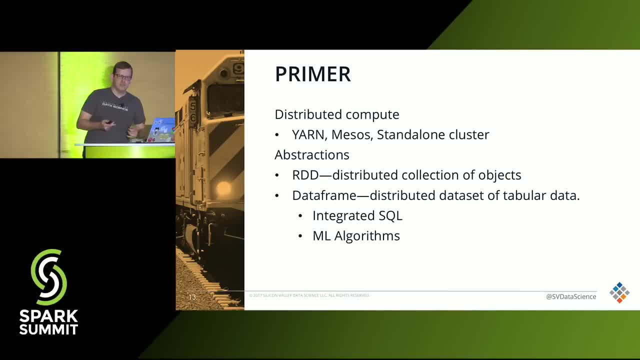 can also work locally on your laptop. It has two main abstractions: RDDs- distributed collection of objects- and DataFrames, which is a distributed data set of tabular data, much like the Pandas data frame. It has the integrated SQL. 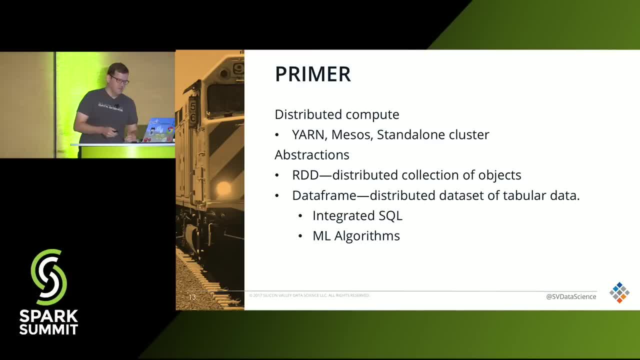 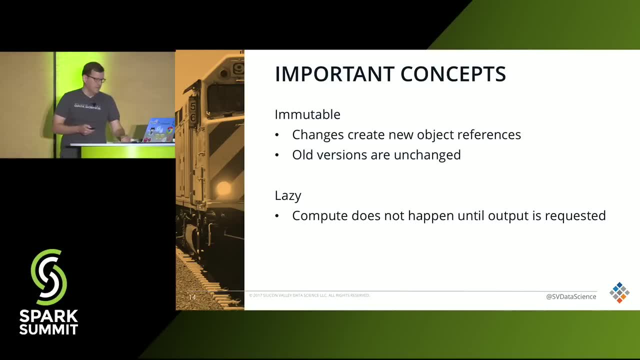 and there's ML algorithms that work on top of both of those. If you've heard a little bit more about Spark, there's also a data set thing, but that's not in PySpark. Okay, So there's two important concepts to keep in mind. 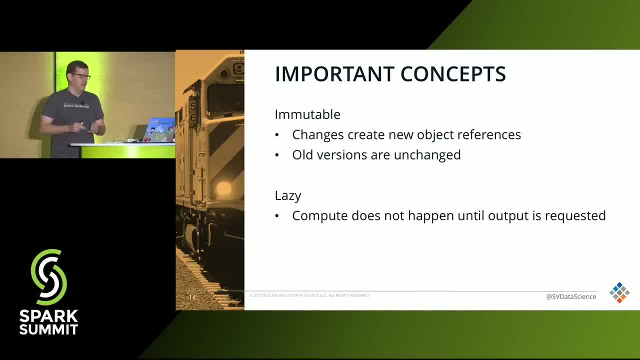 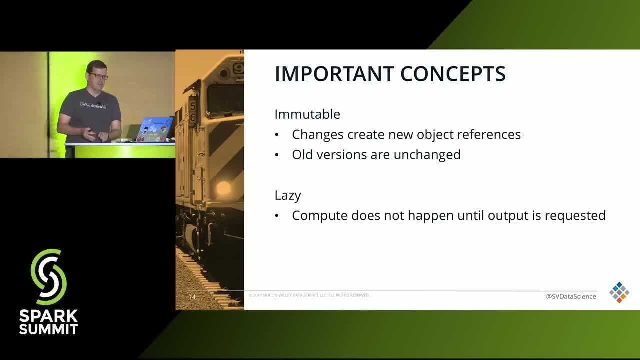 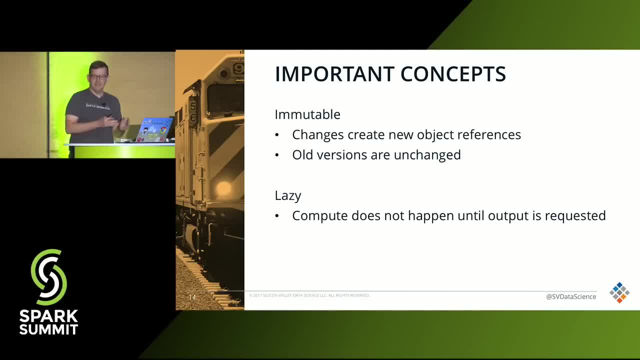 Pandas, sometimes it's hard to know whether or not you are getting a copy of a DataFrame or a view of a DataFrame, and so that's sometimes an area of confusion. You don't have that here, so I think that's a good thing. 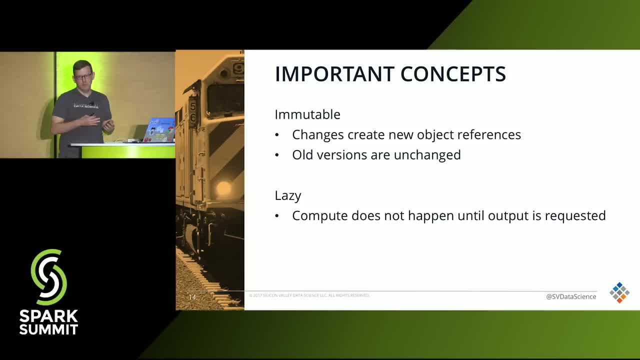 but it does change syntactically a little bit about how you interact with the DataFrames. Another thing is lazy evaluation and that means that the things that you are asking it to do to manipulate your DataFrame don't actually happen until you request some sort of output. 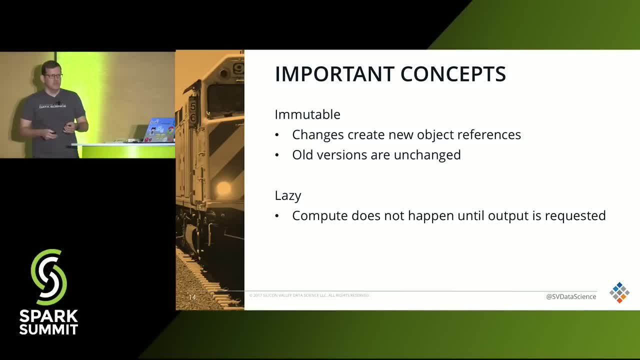 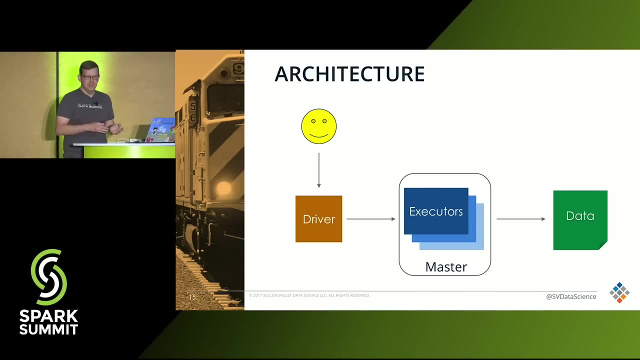 But this is good because it allows PySpark to fuse together the operations that you are doing and do other fancy optimizations to make that all run faster, And just a very, very simplified picture of architecture. so we're all clear on terminology: You, the user- that's the smiley face there. 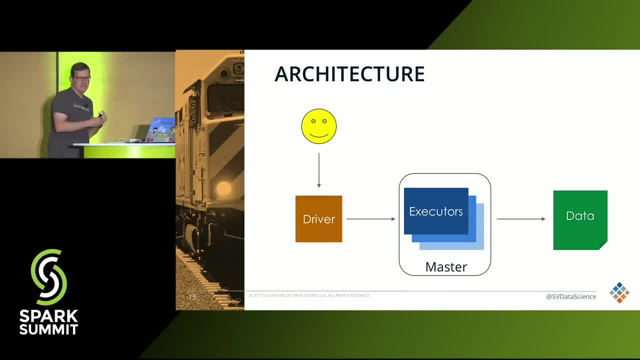 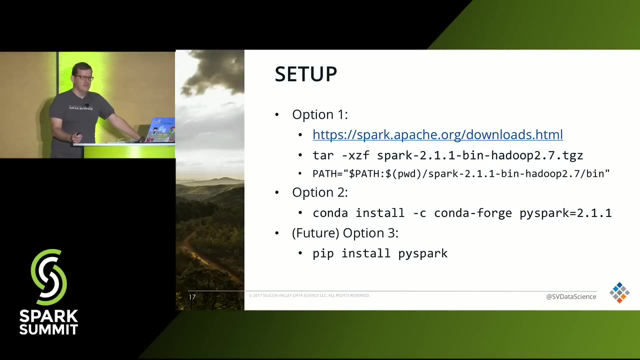 interact with a driver, which then, in turn, operates with executors that run on your master, that operates on your data. okay, All right. so how do we get up and running with PySpark? So there's a few different ways. 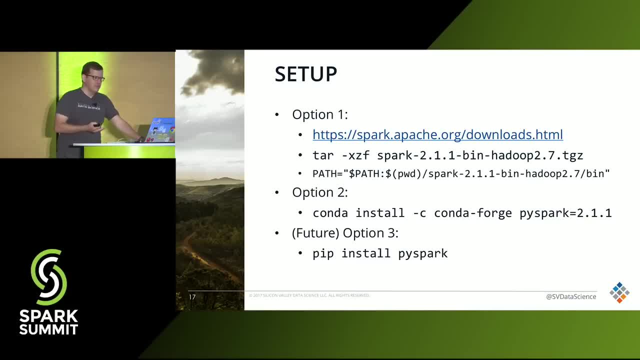 The first way is go to the Spark website, go and download it And add the bin directory to your path. The second, more recent option is if you are a Conda user. which, how many people use Conda? Excellent, excellent. 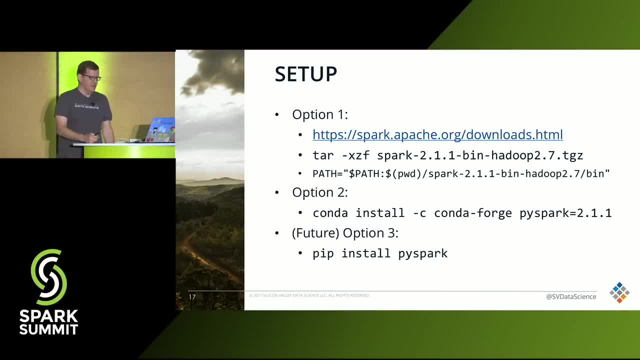 You can use Conda to install it. It's on CondaForge Optionally. make a new Conda environment and it works great. In the future- very soon, once some issues are resolved, you'll also be able to pip install it. 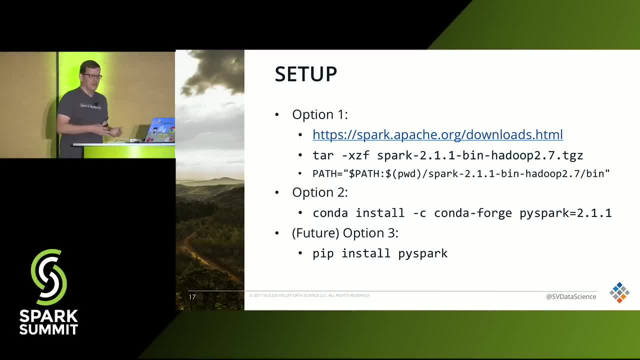 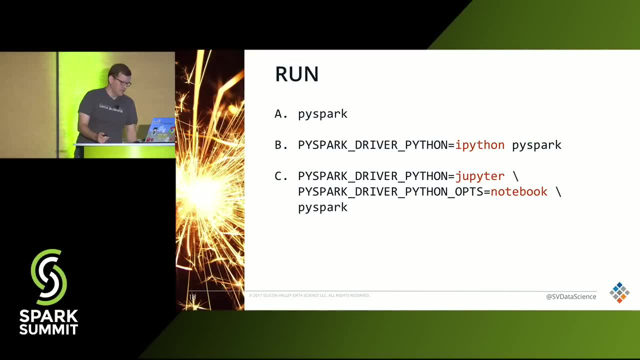 which is great for people that you know. either don't use Conda or don't have the option of using Conda for other restrictions. Okay, and then, once we've done that, it's just a matter of saying PySpark Or, if you want, an IPython shell. 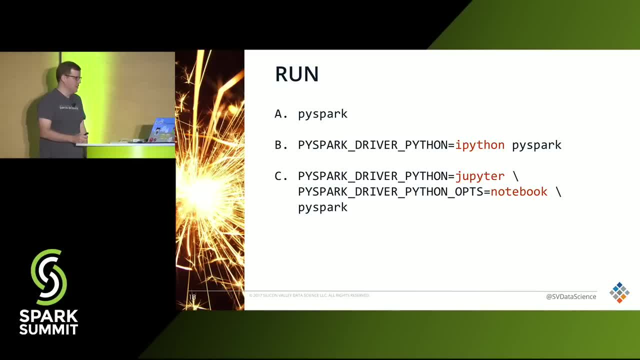 you know a little bit fancier stuff. you can put that environment variable first, or you can add that to your profile. Or if you want a Jupyter notebook, you can add those two, two environment variables and get that to launch when you run PySpark. 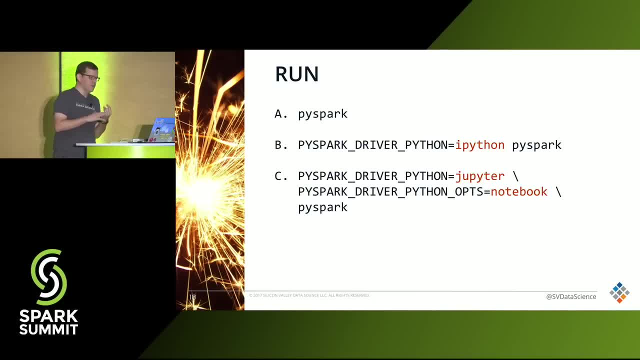 There's other ways of setting it up, like creating a proper kernel spec for JupyterHub or Jupyter. excuse me, If you want to do that and you look on the internet, it's fairly easy. Also, note that this is running in local mode only. 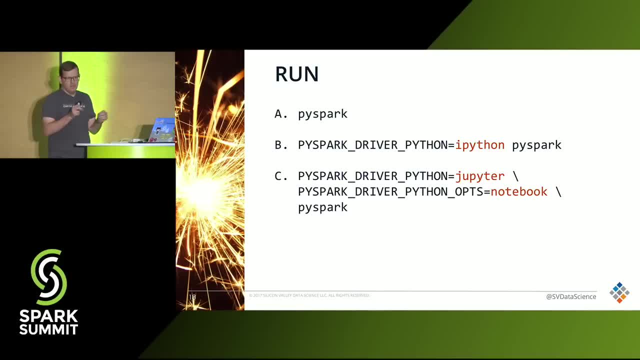 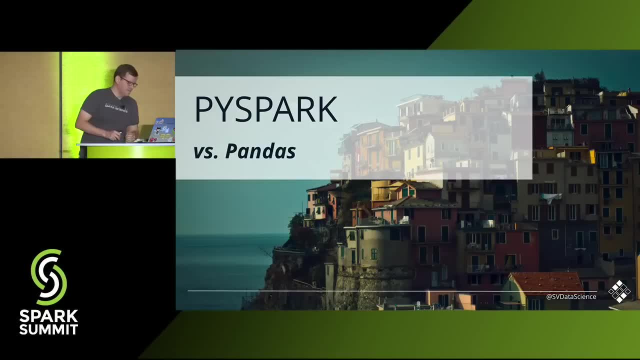 If you want to actually connect to a cluster, you have to add some more options on there and point it to some configuration files. Look in the documentation. All right, so let's compare it to pandas, So probably the first thing you want to do. 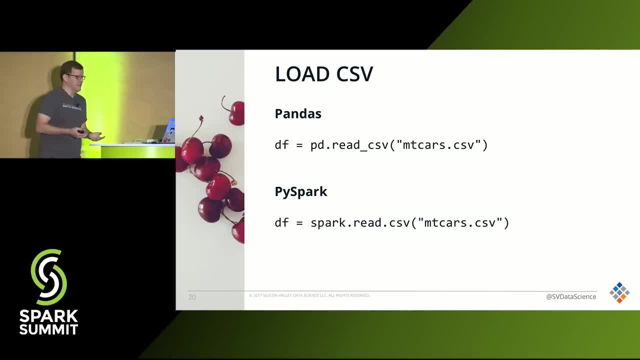 is you want to load in some data. So say, read a CSV, So you know very similar, right Okay? the first example's a lie, right Okay? The defaults are unfortunately a little bit different If you actually want to do this with a common CSV. 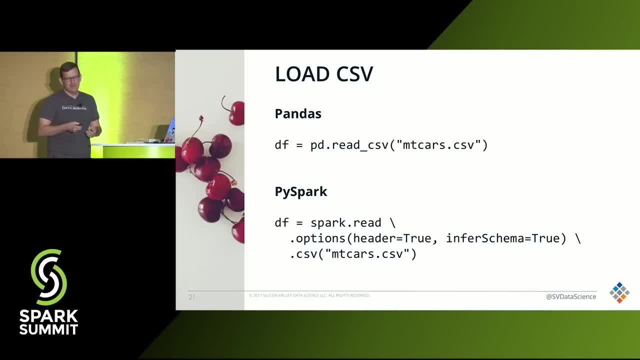 that has a header and probably data types other than strings and you want those data types in your data frame. you probably want to pass in some options to get slightly more sensible handling of those And with all of the data formats that Spark you can give these extra options that you know. 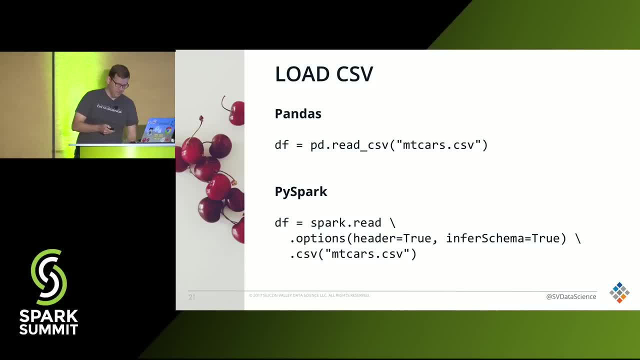 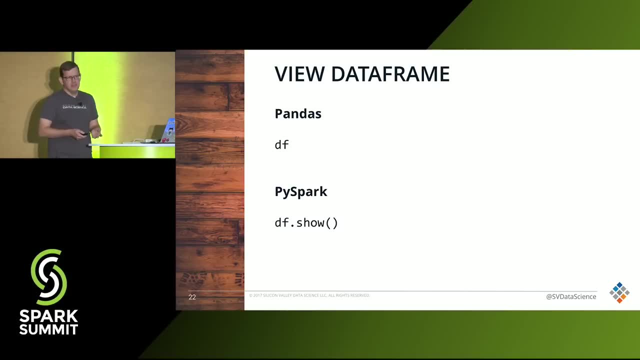 change how that reading in happens. All right, you want to take a peek at it? With pandas it's really easy because the default string representation is: you know the data frame. you know at least some section of it. You have to do a little bit more. 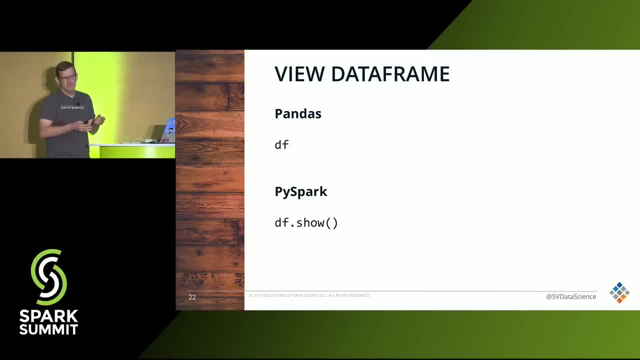 You have to say show, unless you're running on one of the more magic platforms like Databricks. The default string representation of a PySpark data frame is just the schema, not actually the data. So you got to have the show. 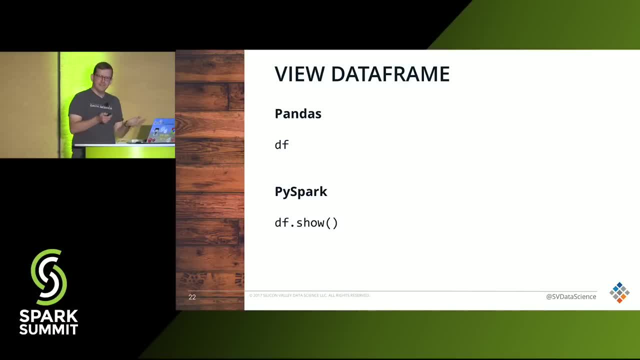 I'm not gonna, you know, throw that on to the further examples, but just keep that in mind. if you're trying to do any of these, All right, and, of course, if you want to just look at a specific number of rows, you can do that as well. 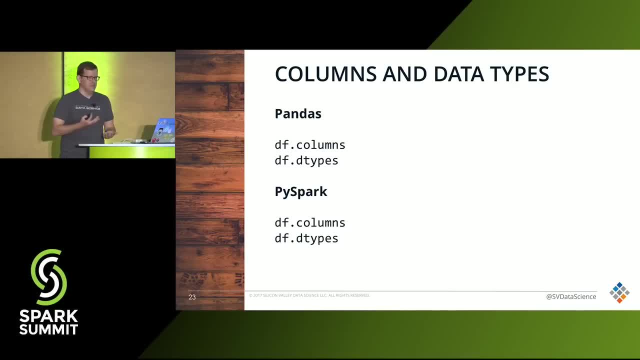 All right if you want to inspect the column names and data types. exactly the same If you want to say, change the names of the columns again because these data frames are immutable. we can't just go make assignments to the column names. 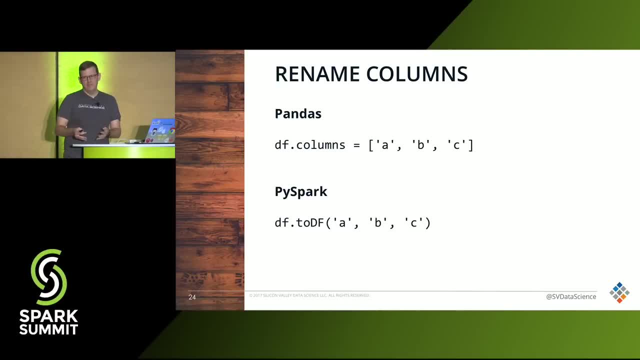 We have to actually create a new data frame with those names. Don't worry, they're not gonna copy anything or do anything. you know intense here, It's just changing some metadata in a new object. but it is a little bit different. 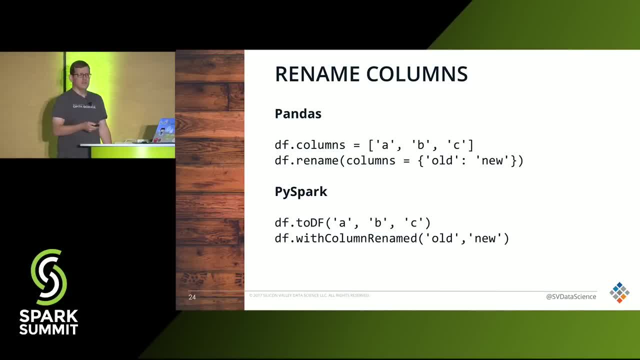 You can also rename individual columns as well, although only one at a time. If you want to drop some columns again, very similar, We'll note that you don't have an axis concept here. In pandas there's the concept of which axis row. 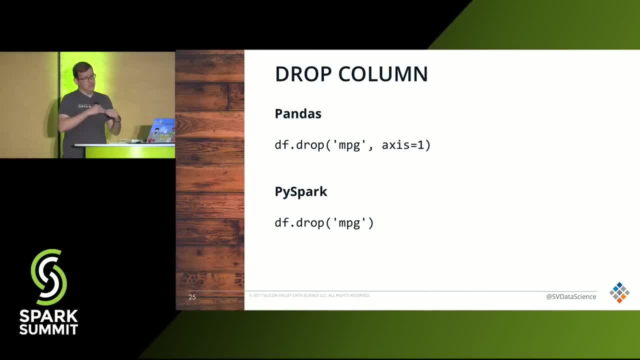 or columns that you are dropping from, because those rows are indexed and you can actually drop like targeted ones. You can't do that in PySpark. That doesn't make any sense, so the only thing you can do is you can drop columns. 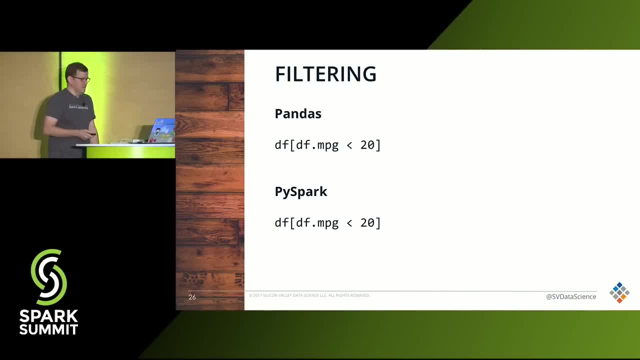 like that. If you want to do some filtering- again very, very similar- You can use the data frame dot column name syntax to refer to your column. you know, make a predicate on that, just like with pandas. Of course, the dot column name approach only works. 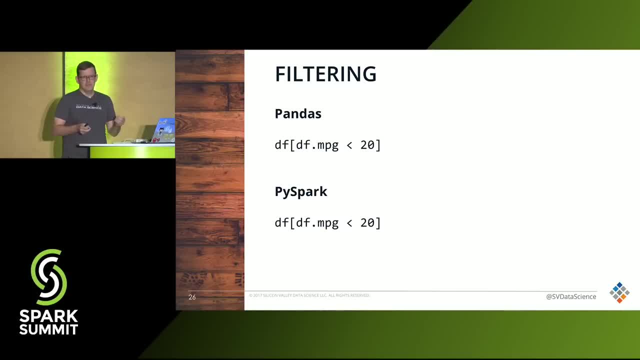 when that's not like a built-in name. so in other cases you may have to use brackets And you can do complex ones just like pandas as well. exactly the same and I will say it will give you equally terrible, terrible error messages. 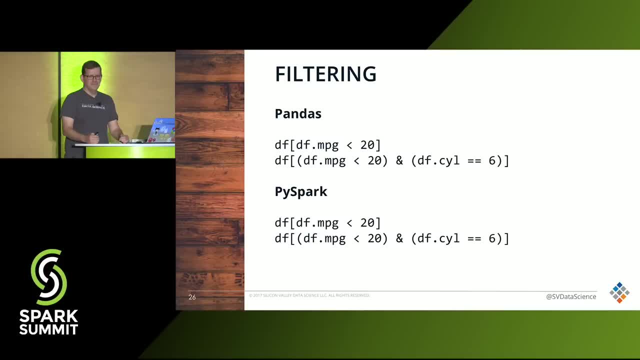 if you forget those parentheses on those compound ones, If you know you get something like that, add those parentheses. Okay, say you want to add a column Again, because we're immutable here. we can't just make assignments, We have to do something else, like this with column: 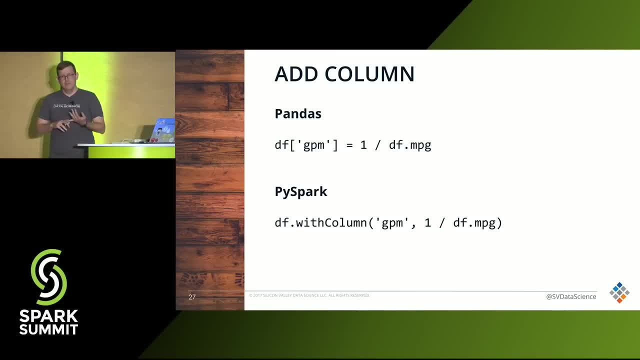 but other than that it's pretty much the same. There are some differences, though, and one that might not be so obvious here, and that is: division by zero in pandas gives infinity and spark it gives null, which is the more SQL-like version of that. 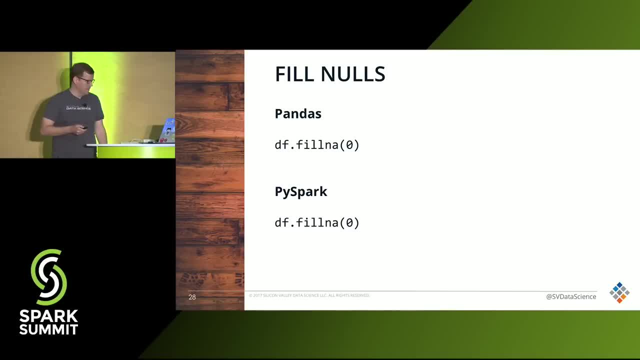 but just keep that in mind. There are some differences. Do you want to fill in As? Also again very similar. although pandas has a lot more options for this, Spark is a little lacking on this. You may be able to recreate some of those more advanced. 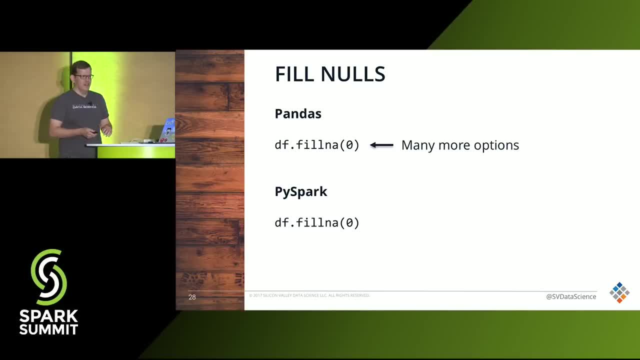 filling options with fancy SQL, but you can do that. You can do that with fancy SQL. but a lot of those things that deal with, say, time series, it's gonna be really hard to do If you want to do aggregation. 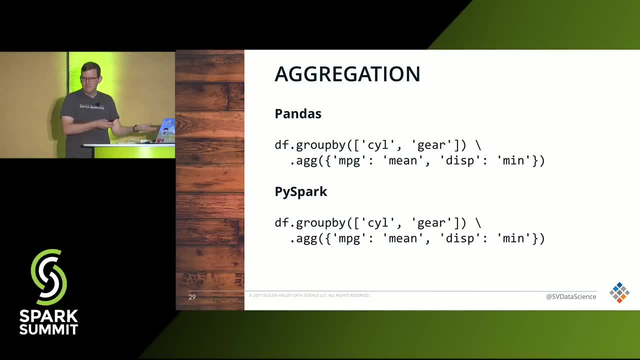 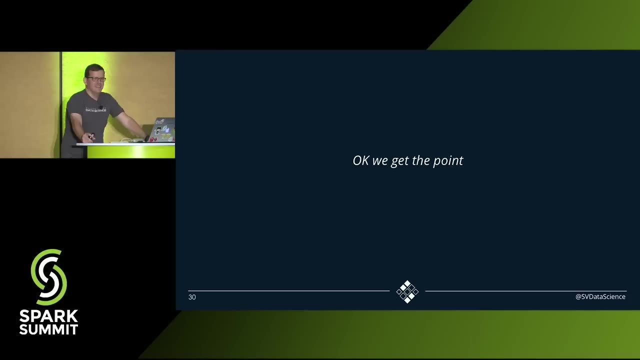 you can do that exactly the same, at least in this syntax option. There are other syntax options that don't line up exactly, but you can do it with the same syntax, like that. Okay, we get the point right. Let's see what else is a little bit. 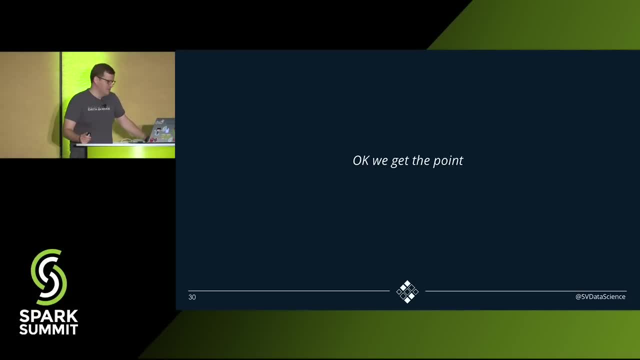 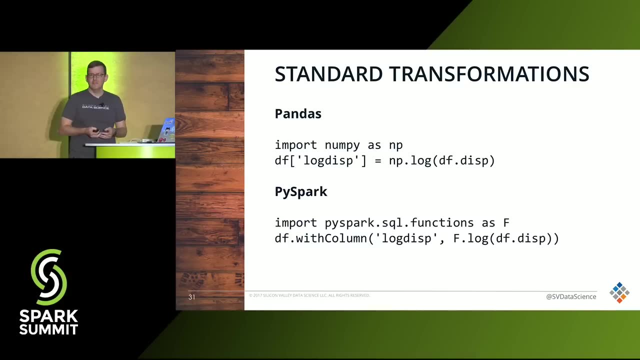 a little bit more different in your transition. Okay, so let's say you want to make a transformation, do some standard transform on a column, Say like: do the log of some value. okay, In pandas your go-to thing for that was to use numpy. 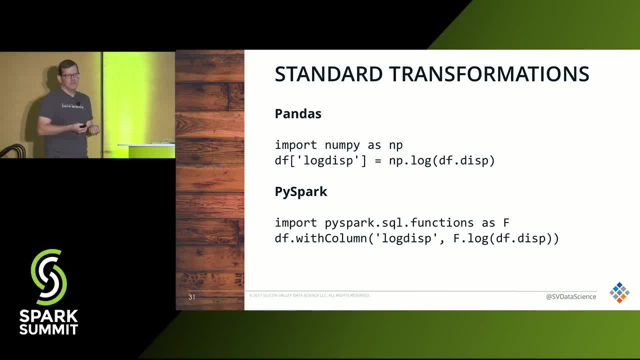 You could use numpy to do the transform in PySpark, but don't. You want to absolutely use numpy to do the transform in PySpark, but don't. You want to absolutely use numpy to do the transform in PySpark, but don't. 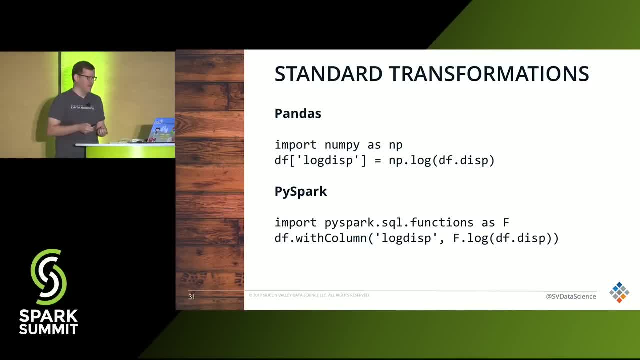 You want to absolutely use numpy to do the transform in PySpark but don't One of the built-in functions in PySpark. So import this pysparksqlfunctions, you know, give it some short name and you're gonna reuse it a lot everywhere. 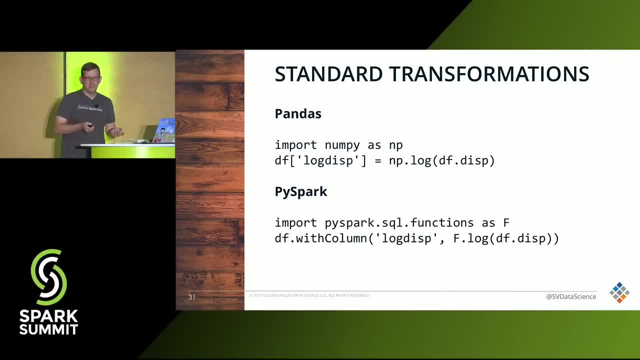 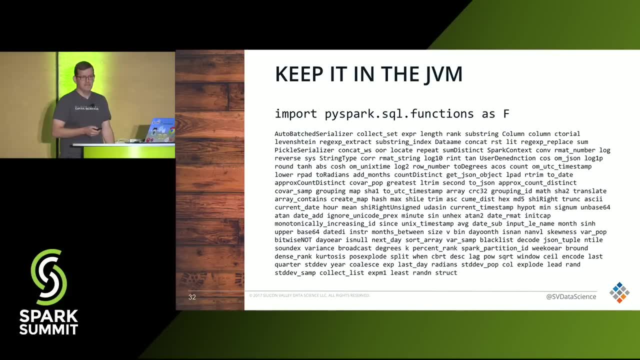 And it's going to have all these common transformations that you're going to want to do every day, And I mean lots and lots of these. Okay, there's hundreds of them, and there's even some that aren't even in there, but that's a different story. 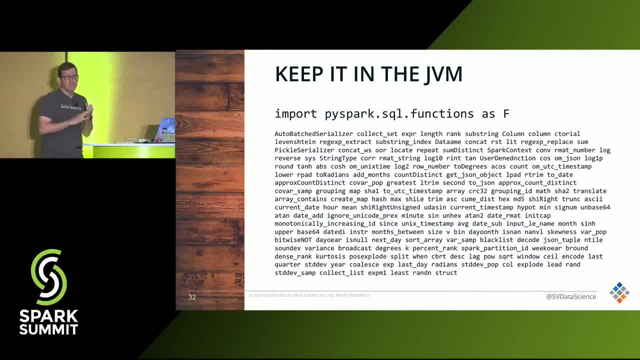 Okay, And I mean lots and lots of these. Okay, there's hundreds of them, and there's even some that aren't even in there, but that's a different story. Why you want to do this is this: keeps the compute that's happening on your data in the JVM. 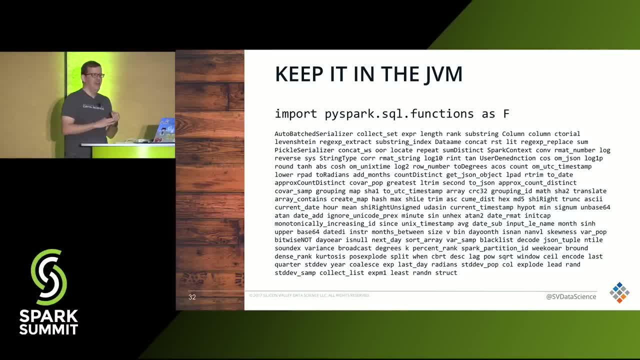 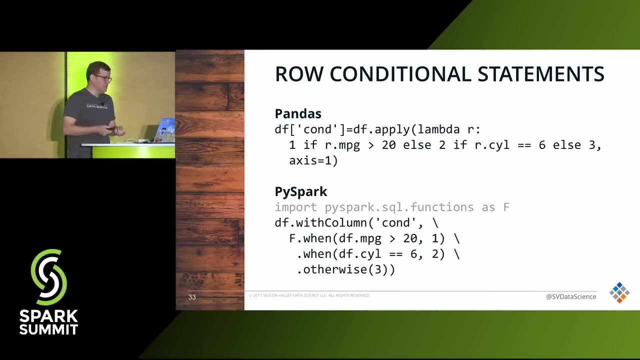 That means you are not actually running any Python at all on your executors. What does that mean? It means it's fast. If you really need Python, it slows it down a little bit, Okay, So just to make the point, you can do some pretty complex stuff. 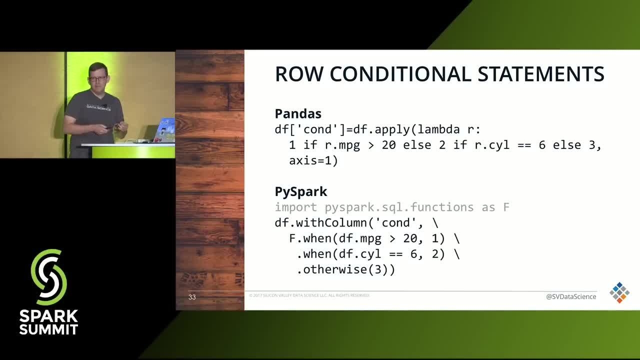 with those built-in functions Like, say, you wanted to apply some complex predicate to each row? Well, you can do the equivalent of that in PySpark using those functions. There's a win that can be chained. basically, if else, if else conditions. 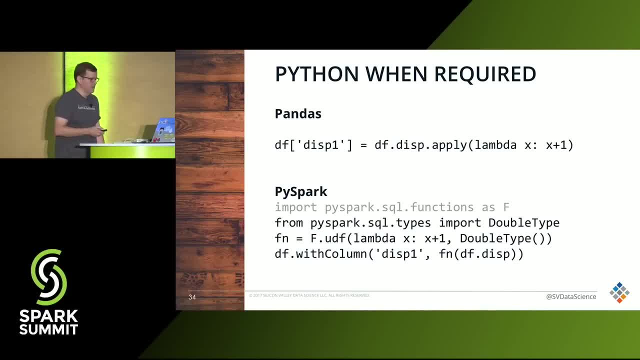 and do the equivalent of that, But sometimes you really just have to apply some Python And if, if you want to. I mean, obviously this isn't a really valid example and we're just adding one but pretend that's more complex. 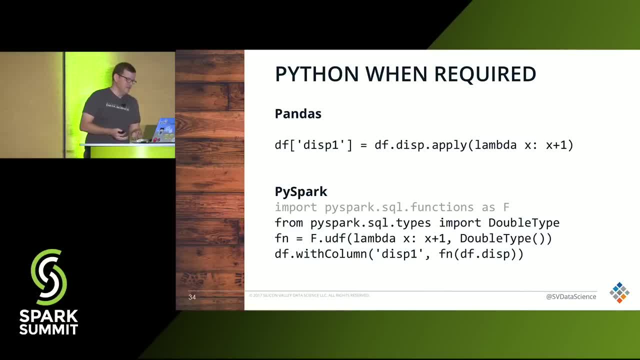 Okay, And we want to apply that to the some column in our data frame. You can register it as a UDF, as a user-defined function. Give the return type of that UDF And it's very important that this is actually. 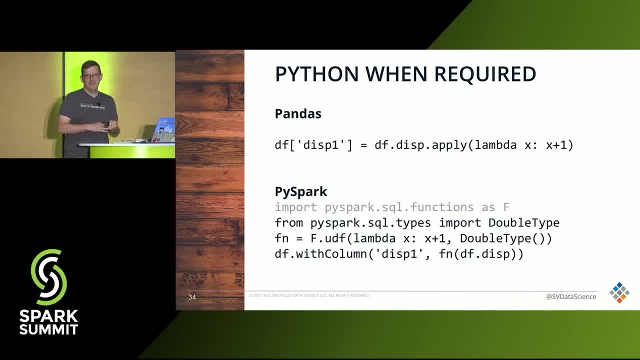 the correct return type. Otherwise your UDF will just give you null every time- Sort of sad- And then you can apply it just like any other function in there. It is important that your UDF be deterministic. That is because Spark might evaluate it more than once. 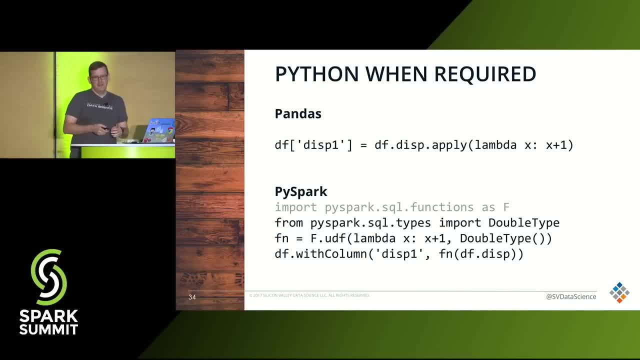 or less than once for each of your rows. It might, it may do optimizations where, hey, I'm going to apply this same function to the same value a bunch of times and only do that computation once. So it has to be deterministic. 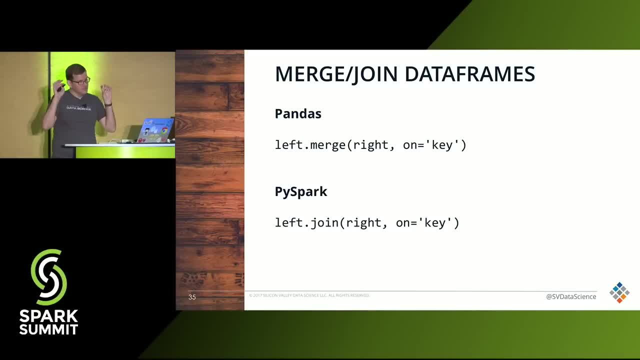 Okay, Say you want to do some join up or merge in the Pandas vernacular some data frames. The terminology's a little different. In PySpark it's only join In Pandas. if you recall, join is for when you want to do a merge on a common index. 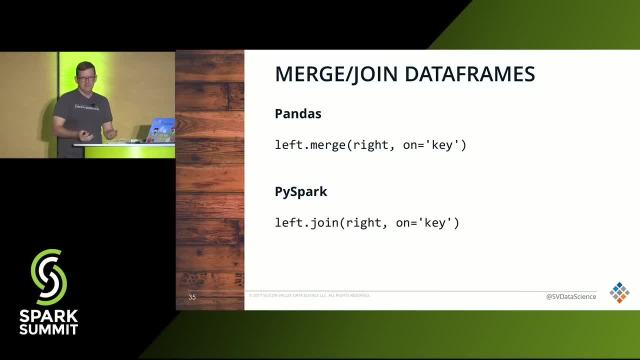 You don't have indices, so there's not that difference, It's all just joins. And if you want to join on, say, your left and right key's a little bit different name, you can do that just like before, but it's a little bit different syntactically. 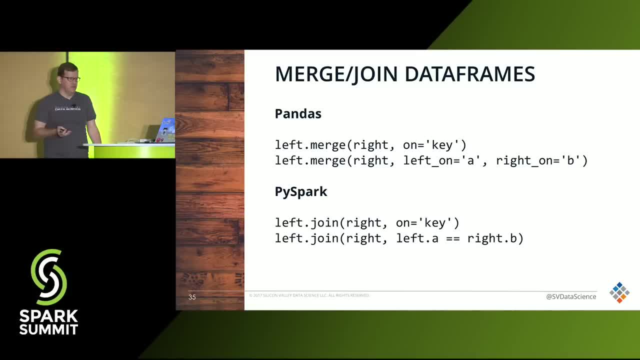 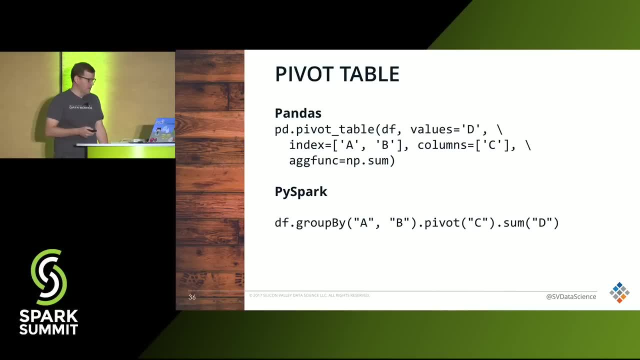 And of course they all support left right, full outer joins, defaults inner join of course, But it's all the same. Quick plug: you can also do pivot tables, just like in Pandas. The syntax is a little bit different. 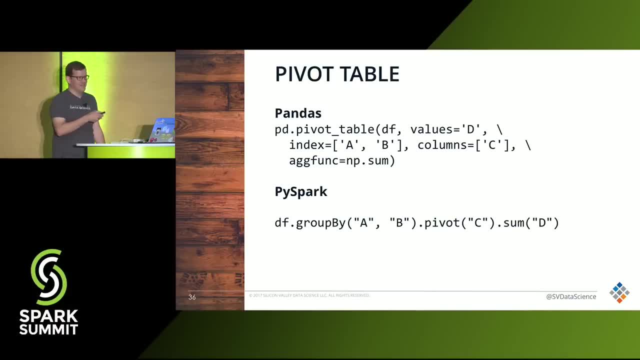 Yeah, I only plug that because that's one of my contributions. so Okay, summary statistics. This is something that you want to do all the time on your data: when you get something new You do describe. Well, you can do that in PySpark. 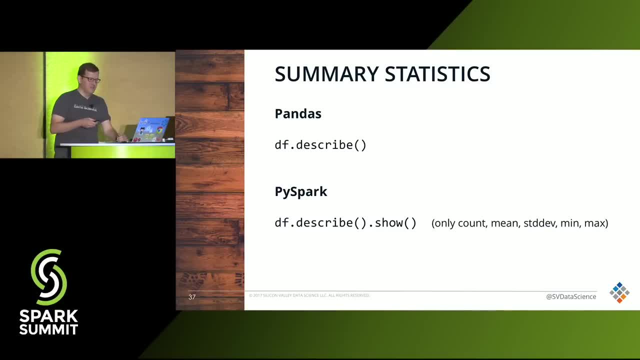 You're gonna get a lot of the same things, But unfortunately it's only going to be the main ones of count, mean, standard deviation, min max. You don't get the quartiles. You can get the quartiles, just takes a little bit more code. 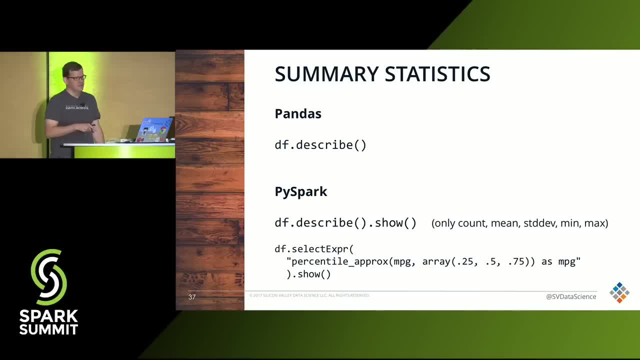 You can use the built-in function percentile of procs, which is built-in, but unfortunately it's not in that functions import that we did earlier. Like I said, there's some additional SQL functions that are built-in that are not in that list for some reason. 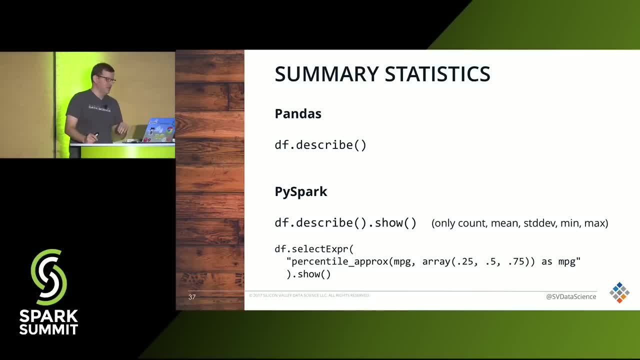 But you can do it as you select an expression and you put in that SQL expression of percentile of procs, the name of your column, an array of the percentiles that you want, In this case the 25th, the 50th and the 75th percentile. 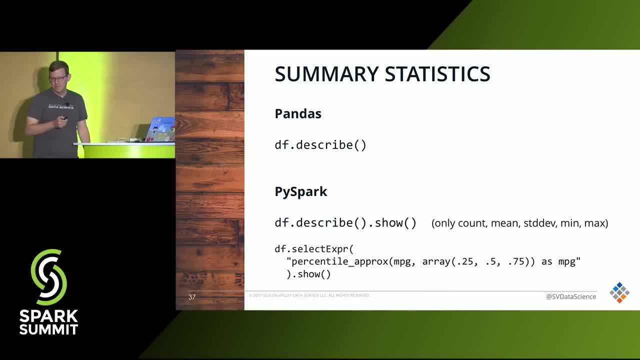 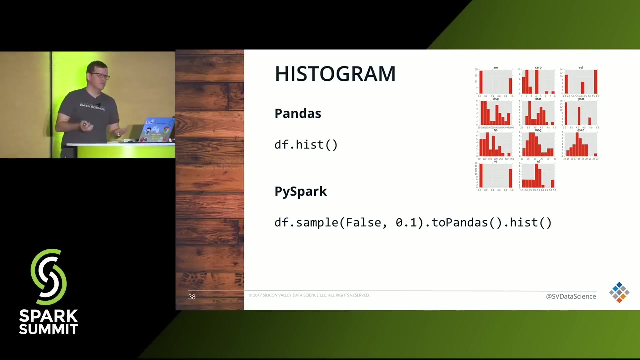 Yeah, yeah, I mean, you can do that fairly easily as well. Let's talk after Count a name, Okay, histograms. Pandas makes it really easy to graph things. PySpark unfortunately doesn't, But you have an escape hatch. 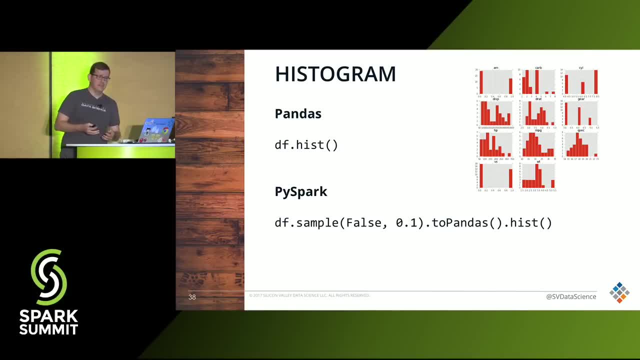 And that is the wonderful to pandas method, which converts your PySpark data frame into a pandas data frame, And then you can do all the things that you could do in pandas before. However, you're not going to want to in general. 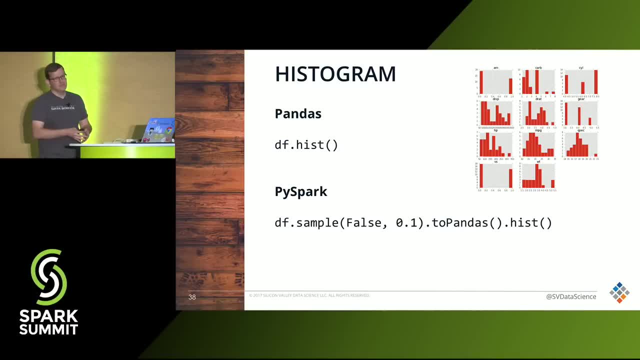 convert that all over, because probably your PySpark data frame's something that's huge And if you tried to put that all in memory you'd run out of memory. So generally you want to do a sample or a limit before you do that, so that you know you don't have to do that. 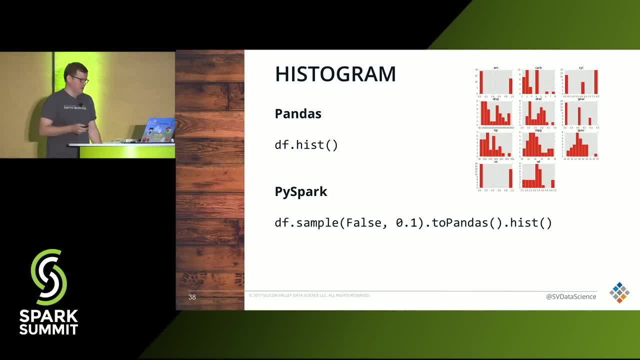 So that you don't have to do that. You don't have that problem. Also, if you really really want, you can do exact histograms. Probably don't need to. If you ask a statistician, they're gonna say no, you don't need to do that. This is good enough. in general. It's okay. Okay, SQL Pandas does not have SQL support. There are third-party libraries like Yhats Panda SQL, but it's built upon SQLite, which, if you're not familiar with it. 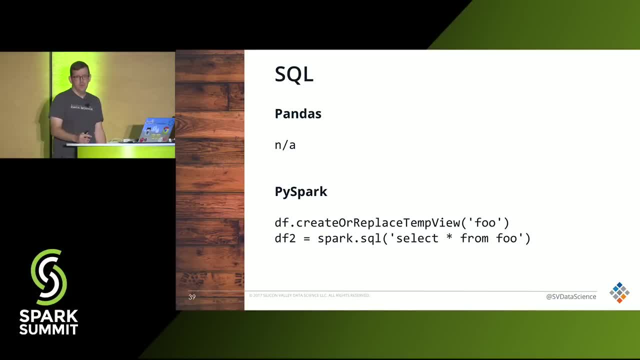 is a bit more limited in SQL syntax support, Whereas PySpark has very, very good SQL support, including, like analytical window functions and all that kind of fancy stuff. So there's lots of cool stuff you can do, And the other part is you can switch back and forth. 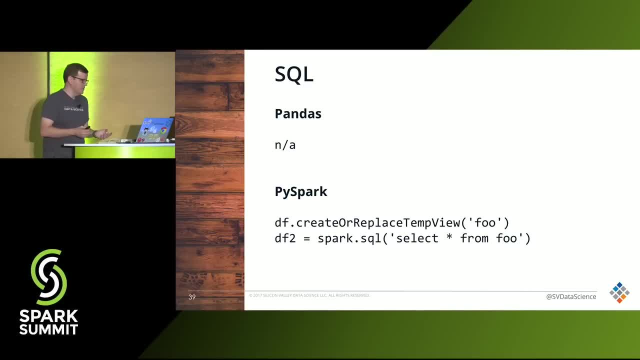 between SQL and data frames. That is, and like in this example, you're not going to want is like in this example: okay, we are registering a table. so basically, I have a data frame, I give it a name that can be accessed in the SQL world. 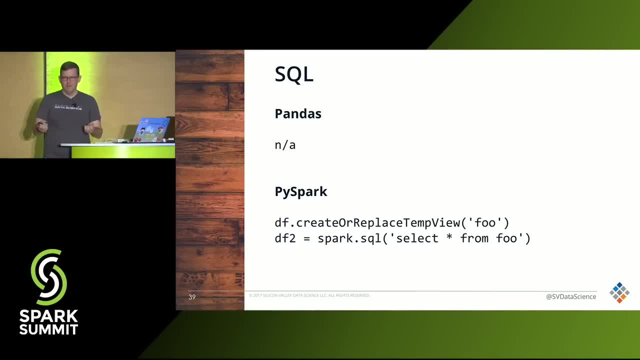 I do some SQL select statement. I'm not really doing much here, but you could do any arbitrary statement and you can assign the result of that SQL to a data frame. Remember, this is lazy, so it's not actually doing anything yet, okay. 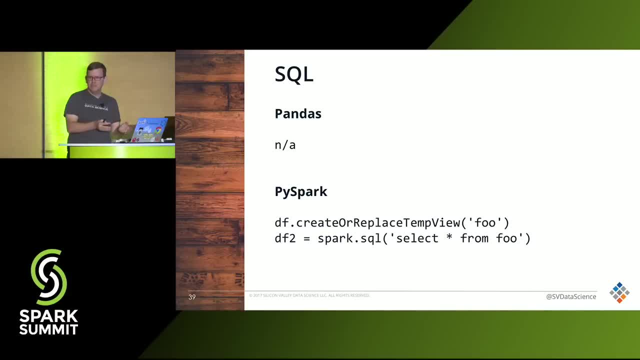 It's just making that as a reference and you can then continue to operate on that data frame just like any other data frame, and it's going to fuse all those operations together at the end when you actually try to output it, because it's all really one unified API. 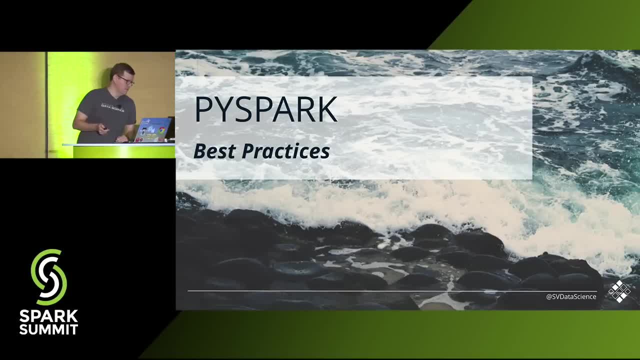 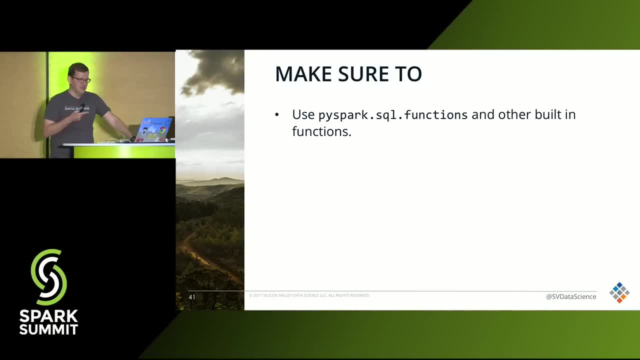 All right, so let's talk about some best practices. Okay, make sure to use those built-in functions. They will make your life a lot better. yeah, because it saves a lot of time. Okay, use the same version of Python and all of your packages on the cluster. 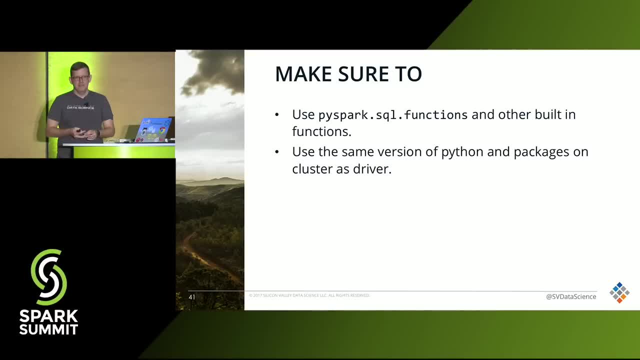 that you're running on as the driver. okay, If you don't ensure that this is the case, you can run into all sorts of crazy problems when you're actually, you know, go to run that Python code that has to execute on the. 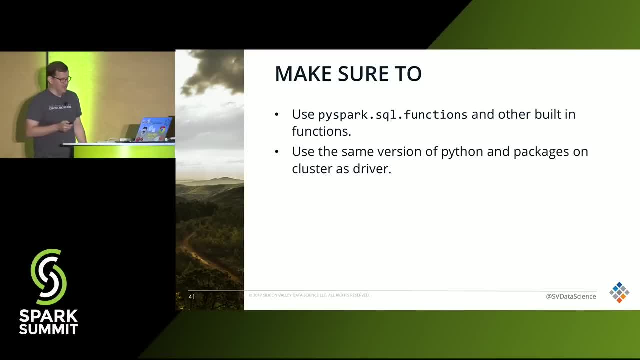 on the cluster and things just don't work for some reason. It's, it's a pain. So one way to ensure that is to use conda environments, For example. you can, you know, create a conda environment, you know. 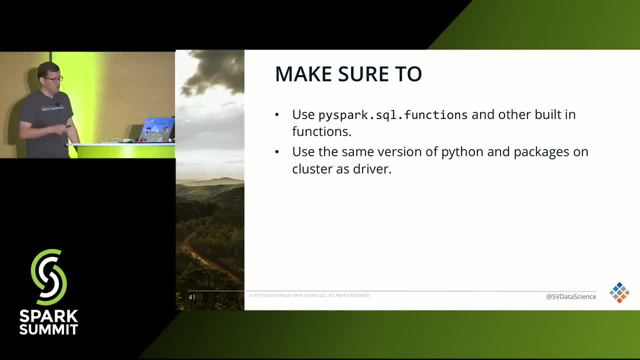 save it, export it out and, you know, make sure that you have that same one across the cluster. Check out the built-in UI for Spark. It's got a lot of information about what's running and it can help you know. 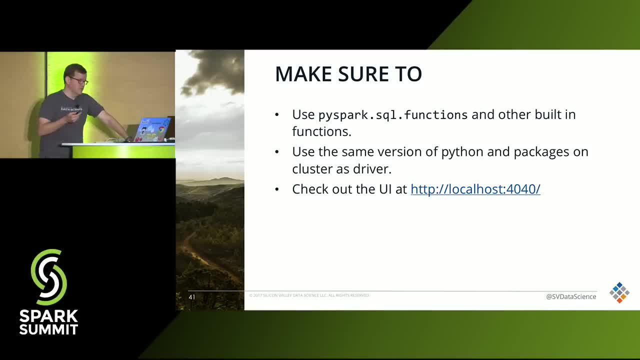 debug some instances where you know things aren't working out right. If you're running this on a cluster and you want to do notebooks, you may want to learn about SSH port forwarding. This can allow you to run notebooks off on a cluster. 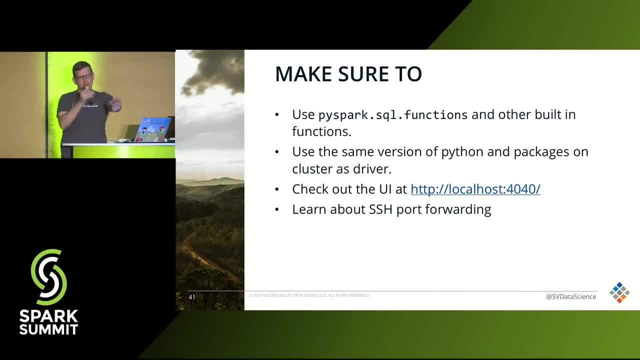 when all you have is SSH access to it. You can forward those ports over to your local computer and still access that notebook. Another way to go about this is JupyterHub, if you have, you know, more people and someone to set it up. 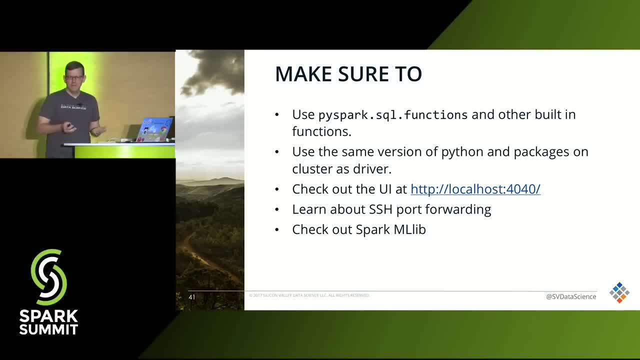 Check out Spark MLlib. It's sort of the equivalent of scikit-learn on PySpark. Gives you all that- machine learning libraries at scale And finally read the fantastic manual It's. it's really not that bad. It's not as great as as. 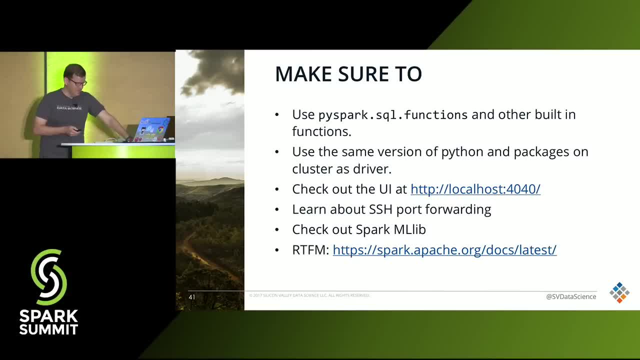 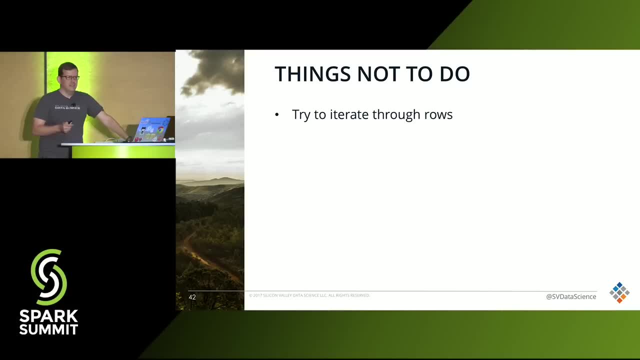 uh, Pandas, But it's. it's there, All right. What not to do. Don't try to iterate through all of the rows. This works perfectly fine in in Pandas. It's not the most efficient thing. 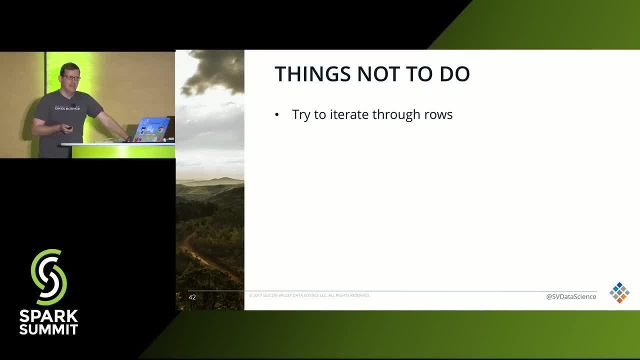 but you know it'll get the job done. You can't do that in Spark. It just doesn't work. When you're writing these things as a script, don't make the mistake of trying to hard code a master. Um, do that in the the Spark submit command line. 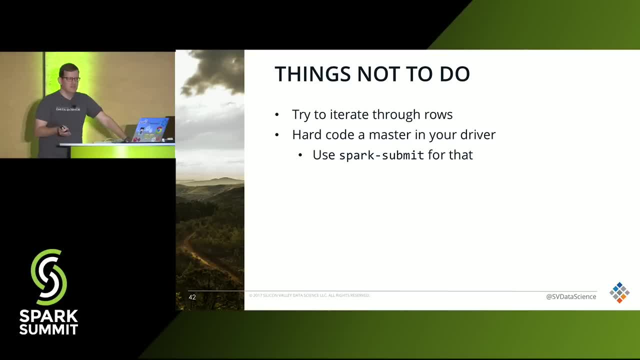 Um, and that then your scripts will be a lot more versatile. You can run it, you know, however you want. If you're going to do filtering um on something that you're converting to Pandas, do it before the conversion, not after. 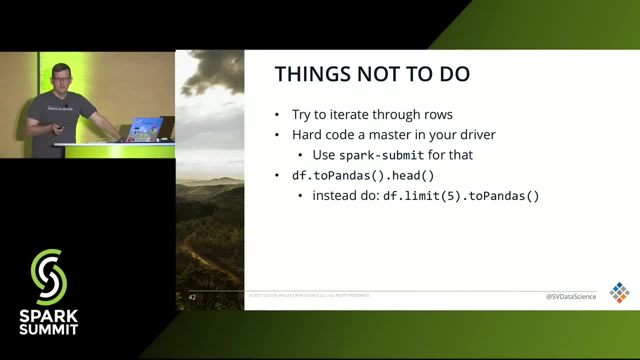 If you, you know, do that first thing, it probably won't run because you're doing the filtering after. Okay, What to do if things go wrong? Don't panic. read the air. Sometimes they're good, sometimes they're not. 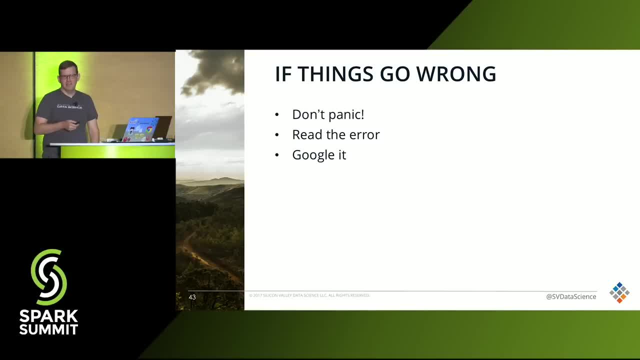 but definitely Google it because someone else has ran into it before most likely. Uh, there's uh active uh stack overflow page uh with the tag Uh Apache Spark that you can search and ask uh questions on. 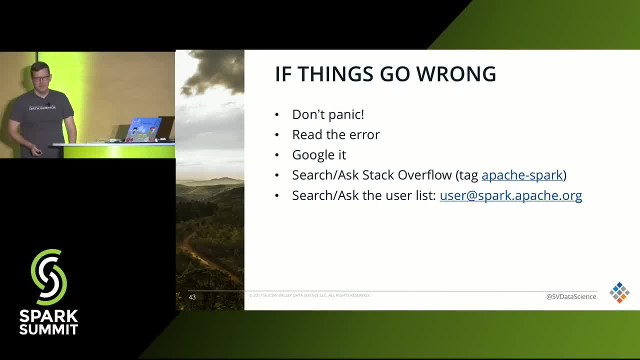 And there's also an active user mailing list that you can search the archive the day before and search the archives of or ask new questions on as well, And if you find something that you really think is a bug, please just go file a JIRA ticket. 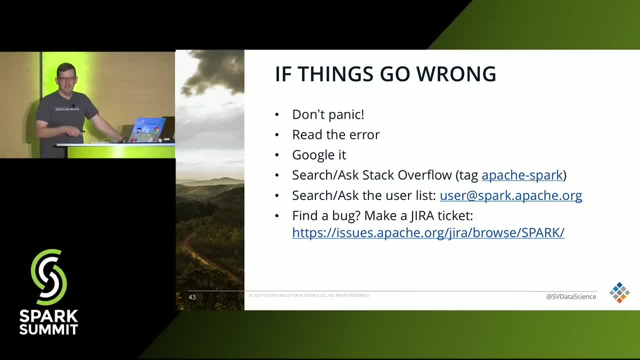 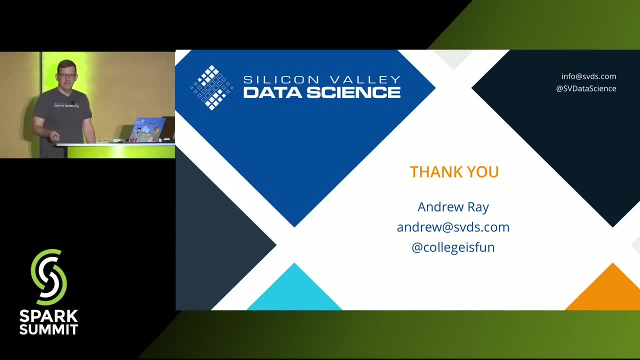 The worst that will happen is someone will say, no, that's not a bug, do this All right, that's it. Remember I have another talk later this afternoon if you're interested in graph algorithms. Thank you, Hi. thanks for the introductory talk. 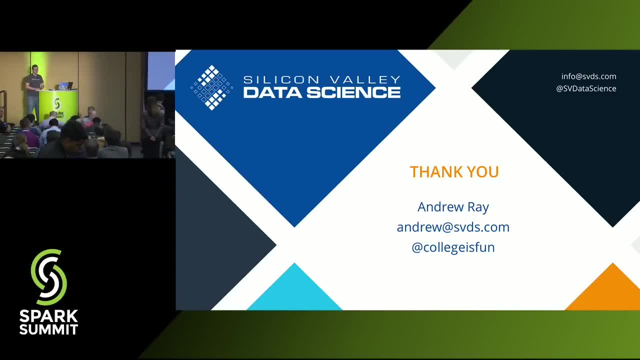 It was very, very useful for me, And I have a question: is there any reason I'm a data scientist? is there any reason I should invest time in the Scala Spark? Yeah, in which Spark? Scala, Scala, Oh, okay. 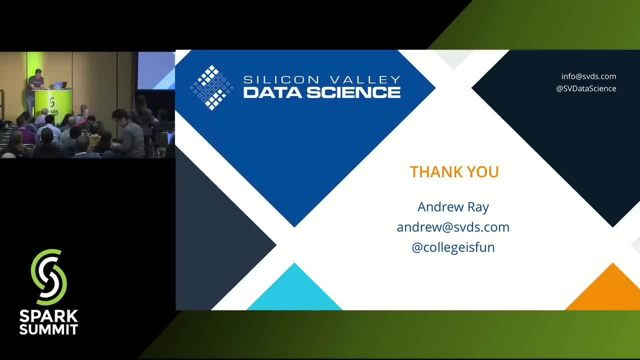 Or I focus my efforts in PySpark. So there's a couple aspects. There's a couple aspects of that. One is preformance. If you care about preformance and you want to do a lot of custom stuff, that's not built-in. 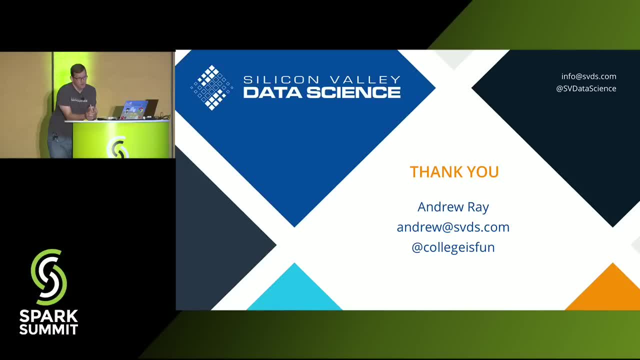 if you're using Scala or Java, you can get a little better performance, But if you're using all of the built-in stuff, the performance is exactly the same because it's actually being executed exactly the same. The second is API completeness. Unfortunately, there are some cases where the Python API lags a little bit behind the Scala API. Like new things are added, like a new algorithm in MLlib is added, but no one added a Python wrapper for it. Sometimes that happens- Not very common. most of the time it's equal. 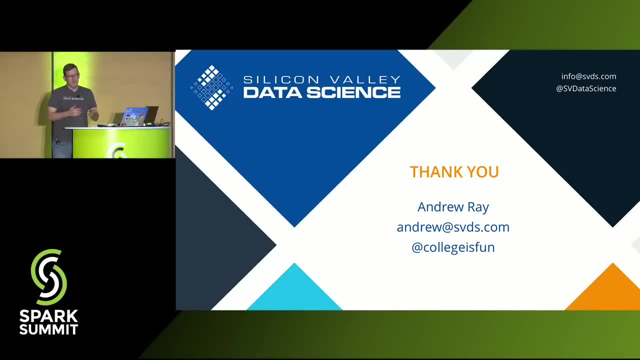 but there are some instances of you know, that Python API is a little bit behind, Usually resolved fairly quickly. So in general I don't think it's worth going to the extra effort of learning a whole new language just for those small little things. 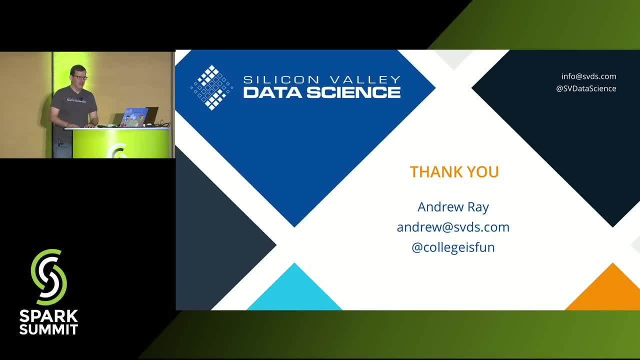 I think it's a much better investment of your time to just learn PySpark and go with that. Yeah, So thanks for the presentation. I have a question about PySpark visualization and correct me if I'm wrong. So are you suggesting that the only way to leverage Pandas? 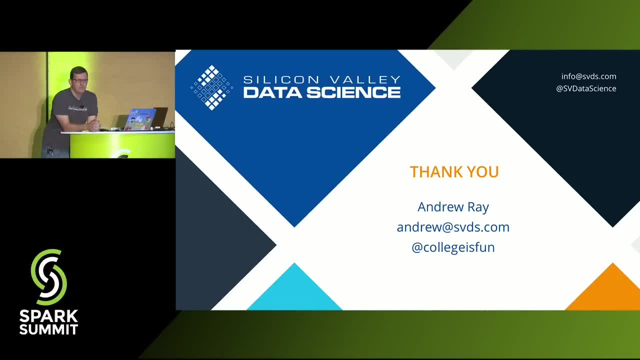 or other basic Python visualization is to do sampling and then transform this to a Pandas data frame, or does PySpark have some visualization libraries? Okay, so there is nothing built into PySpark If you're using some extra tools, like say: 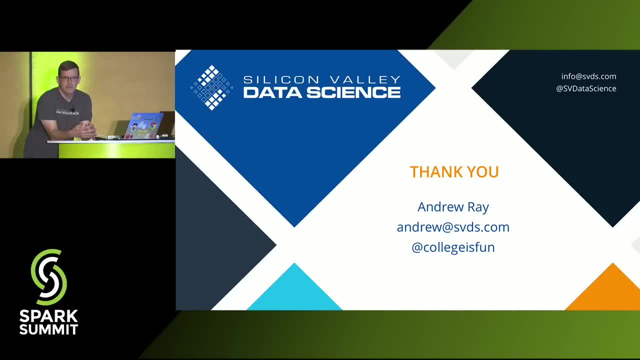 Databricks they have. they have visualizations that can run on your full data frame. But in the general open source sense of just what's included in PySpark, there's no visualizations at all. But generally speaking, when you're looking at a large enough data set, 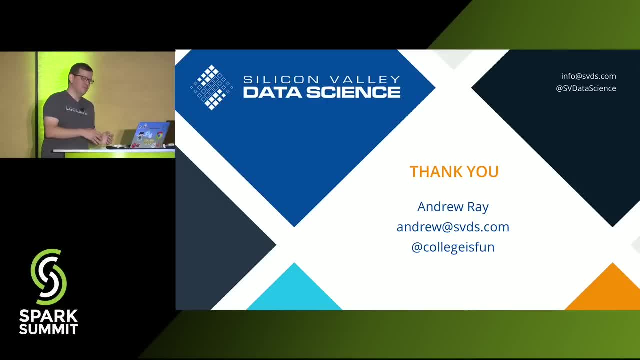 there's not any meaningful difference from a sample of that in the graphical representation and the full data set. This isn't universally true, but for a lot of visualizations there's not like a real meaningful difference. And so I'd say, and it's usually okay. 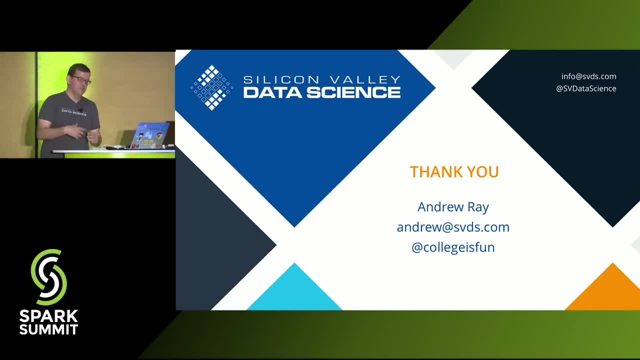 And if the other thing that you can do is, if you want to do this on the entire data set- is you can do those aggregations on your Spark data frame, Because generally your visualization is of some sort of aggregated data, You do those aggregations to essentially shrink it down. 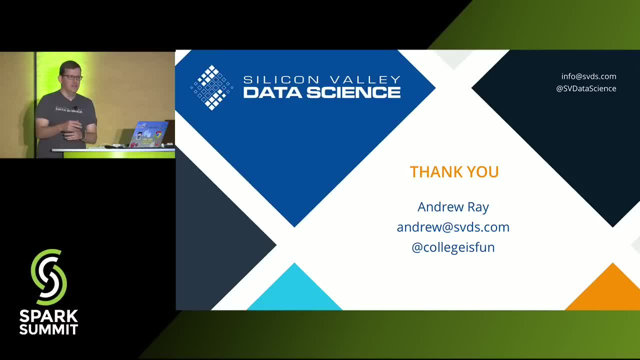 to something that can be done, fit in memory and then do the visualization off of that. Hi, thanks for your talk. I'm new to Python and scikit-learn. Are there any good practices, given that scikit-learn is probably a lot more richer? 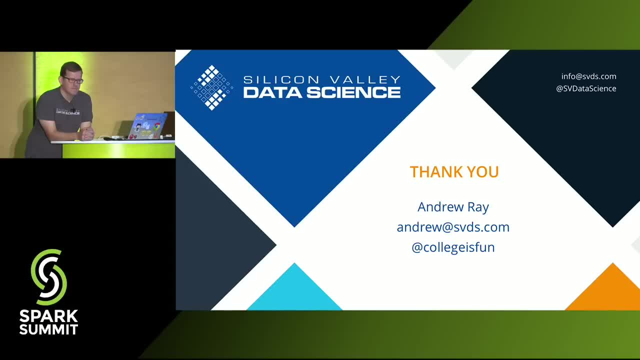 in the terms of what it can accomplish in the algorithms and stuff. So is there a best practice? you follow, that you do some things purely in scikit-learn and then you do some things in PySpark. Well, I'd say, the main difference is: 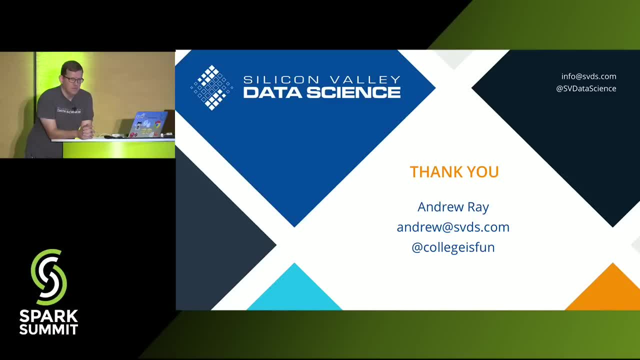 like how big of a data set you can work on If. if I had infinite memory, I would just do everything in scikit-learn, you know, in an infinite compute, right? But there are these realities that we run up against. 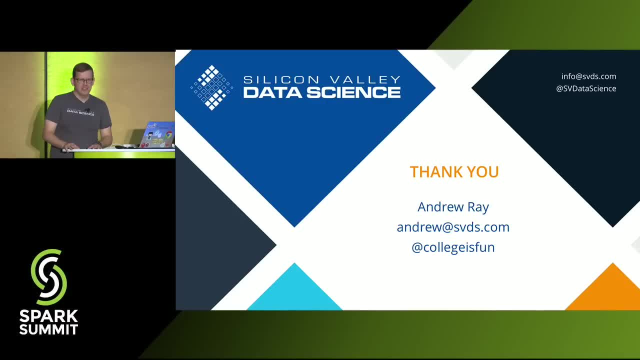 And I think, I think the distinction is really just when it becomes hard to do with traditional tools. that's when you start to look at these distributed solutions like PySpark. So I had a question about writing UDFs in Python And when you write a UDF in Python, 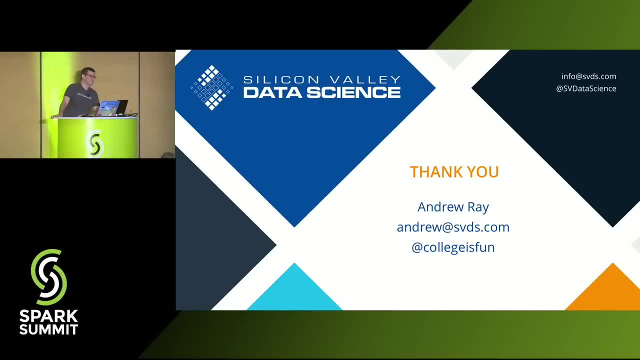 the insight I haven't fully gotten is like you know what sort of what are sort of best practices for writing Python UDFs, Like? the only thing I can think of is like use list comprehensions when possible and these types of things, right. 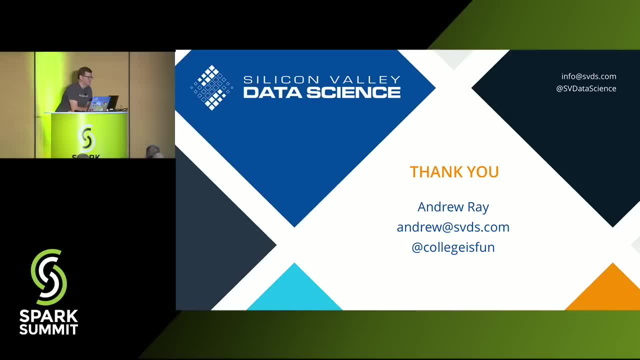 Do you have any thoughts on kind of best practices on how to write a a less painful UDF, like less slow UDF? So one thing that you can do is like if you're doing some sort of numerical thing, just like before.